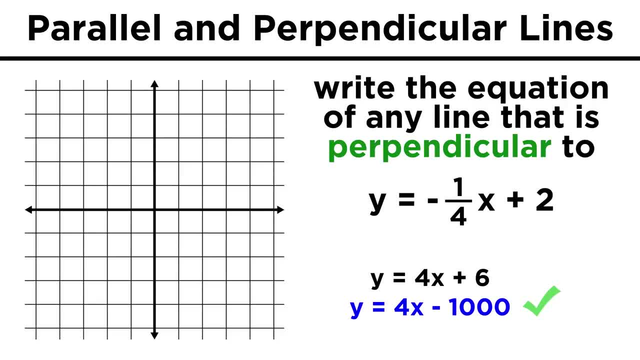 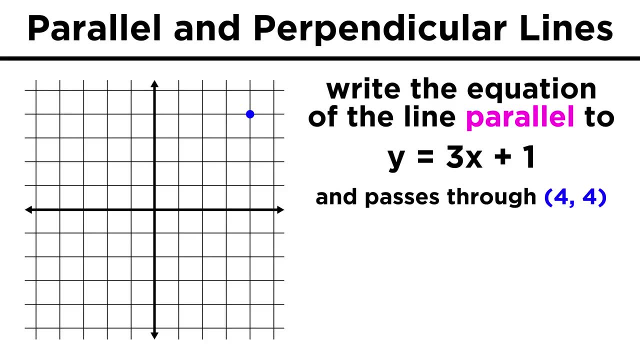 Y equals four X plus six or four X minus a thousand, it doesn't matter. If it has a slope of four, it will intersect this line at a right angle somewhere. Some questions will require that you be a little more specific. You could be asked to find the equation of a line that is parallel to Y equals three. 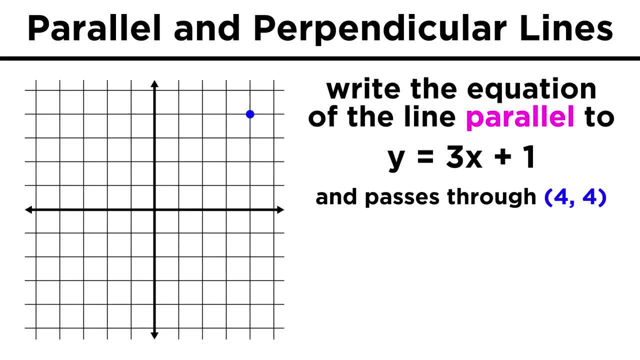 X plus one. Well, if it's parallel, we know it has a slope of three. so Y equals three X plus B. Now we can plug in the coordinates for the one point we know. so four equals three times four plus B, and if we solve for B we get negative eight. so the equation must be Y. 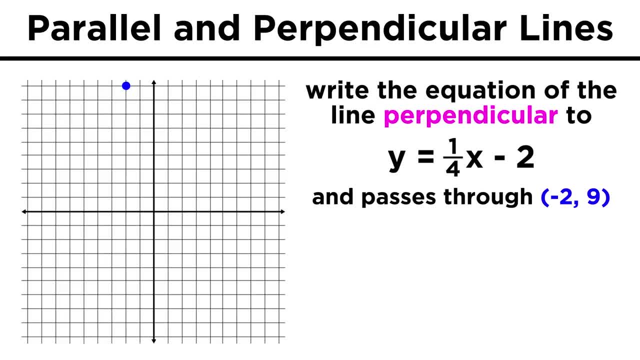 equals three X minus eight. We could do the same thing for perpendicular lines. say, we need to find the equation for the line that is perpendicular to Y equals one fourth X minus two and passes through the point negative two, nine. Well, once again we know we need the opposite, reciprocal, of the slope. 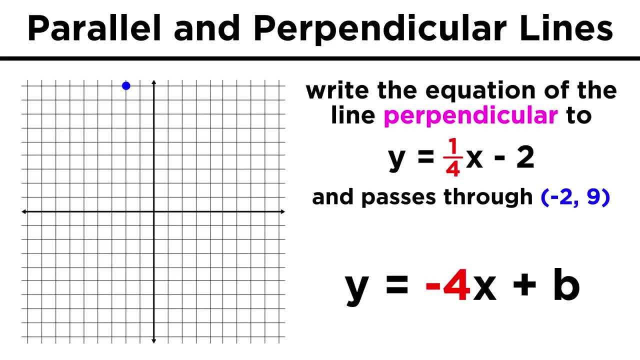 That means one fourth becomes negative four. Y equals negative. four X plus B. We plug in the coordinates of the point we have and nine will equal negative four times negative. two plus B. This product is eight, so negative eight. we subtract eight from both sides and B equals one, so the equation is Y equals. 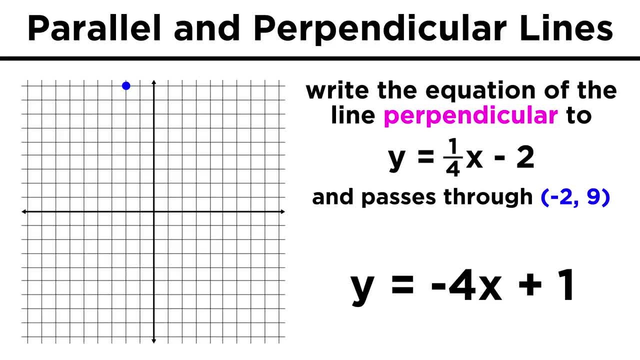 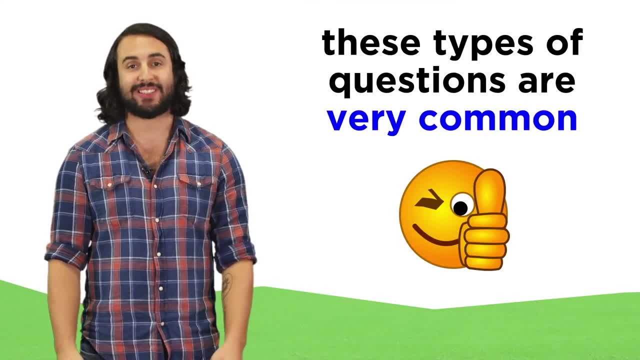 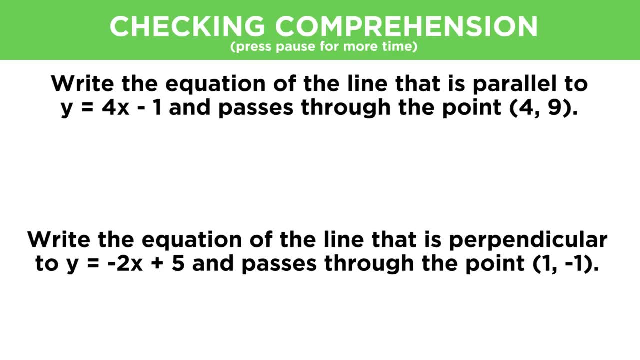 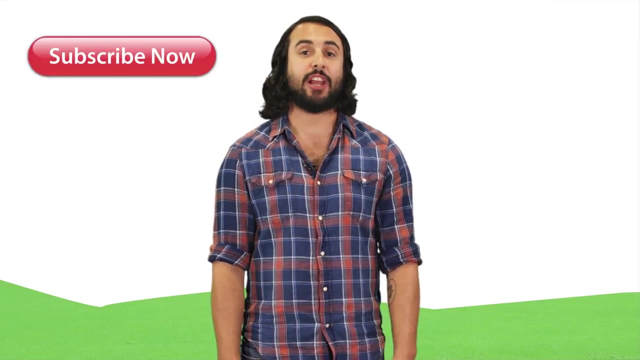 negative four X plus one. None of this is too tricky, but it's important to know these rules as these are extremely common types of questions in algebra. so let's check comprehension. Thanks for watching, guys. Subscribe to my channel for more tutorials. 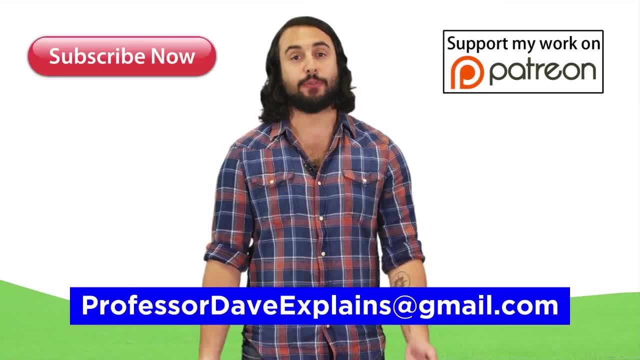 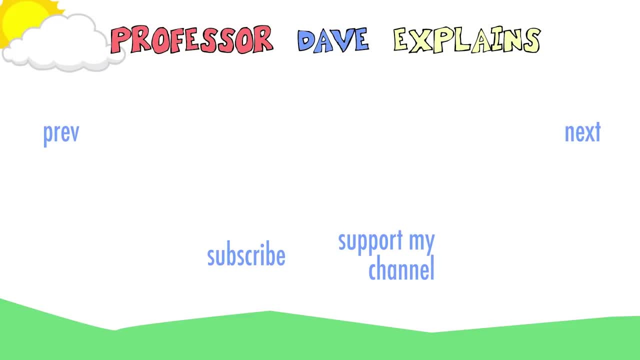 Support me on Patreon so I can keep making content and, as always, feel free to email me, ProfessorDaveExplains at gmailcom. I'll see you soon and have a good day. Bye.